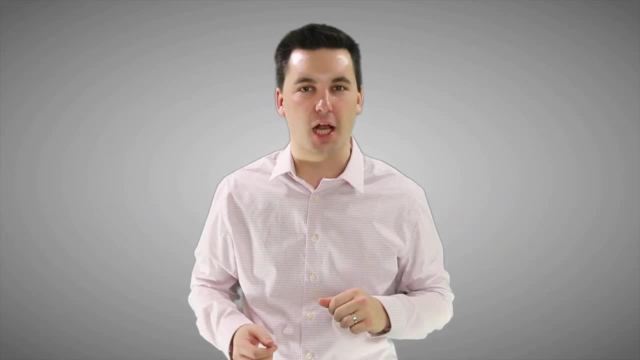 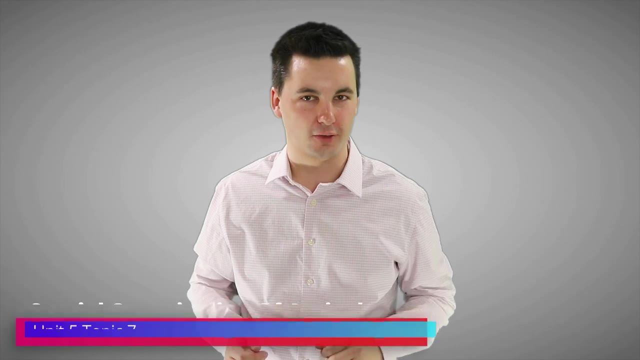 Good morning, afternoon, evening, night, whenever you're watching this, geographers. welcome back to the Mr Sin channel. Today we're going to be going into unit five. topic seven: spatial organization of agriculture. In this video we're going to be highlighting some of 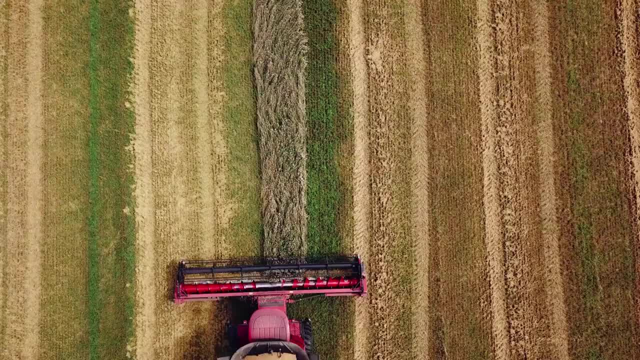 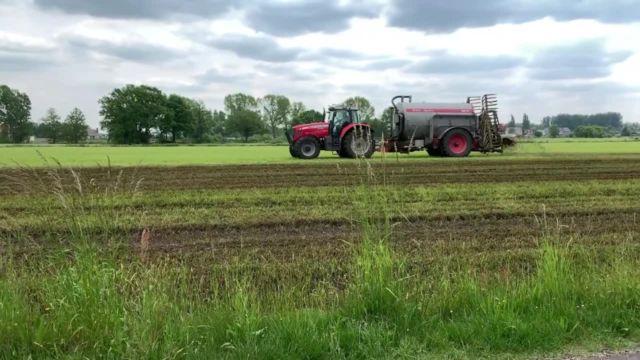 the recent trends that have been happening in agriculture around the world. Thanks to advancements in farming equipment, machinery, transportation, fertilizers and GMOs, we have seen some major shifts in the production of our food. Some of these shifts have been positive. 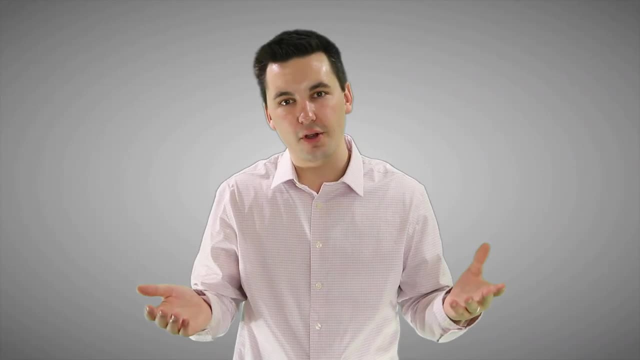 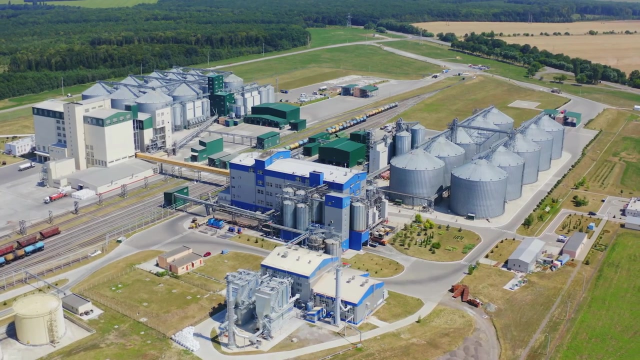 ones and have led to higher food production and specialization, while others have been negative. Since the green revolution, we've seen a rise in agro businesses and corporate farming in the developed world, which has led to a decrease in small scale family farms As agriculture continues. 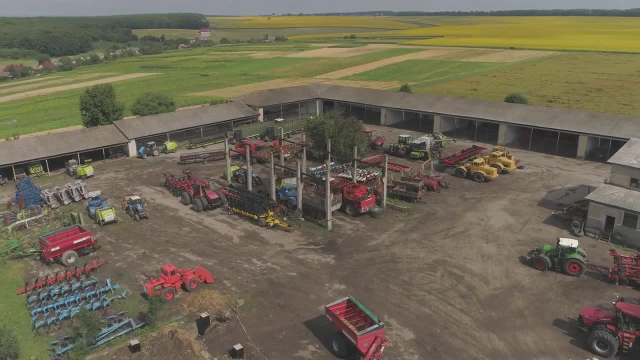 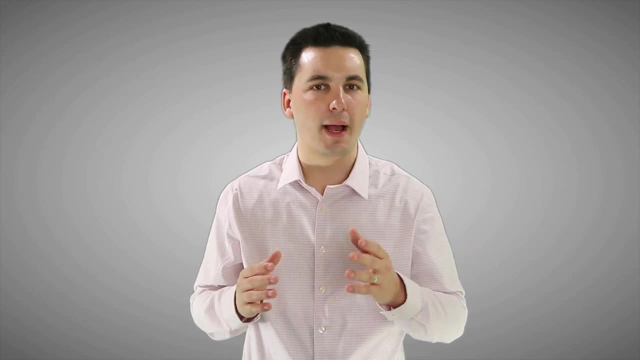 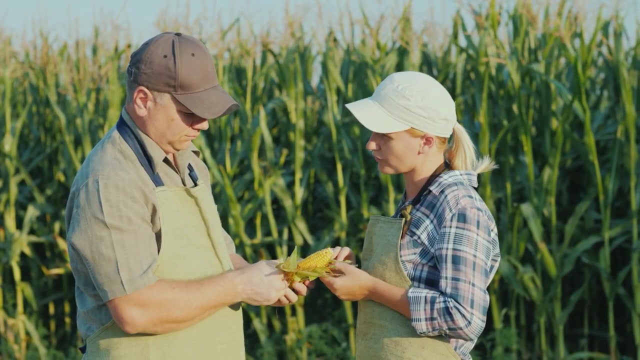 to become more reliant on different types of machinery, it becomes more expensive and more difficult for a family farm to operate. Today, we can see these large scale businesses operating farms around the world. These newly industrialized farms have created commodity chains to help support their growing industry. A commodity chain is a process used by companies to gather. 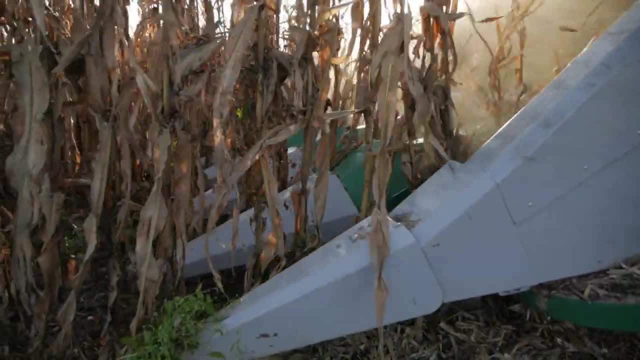 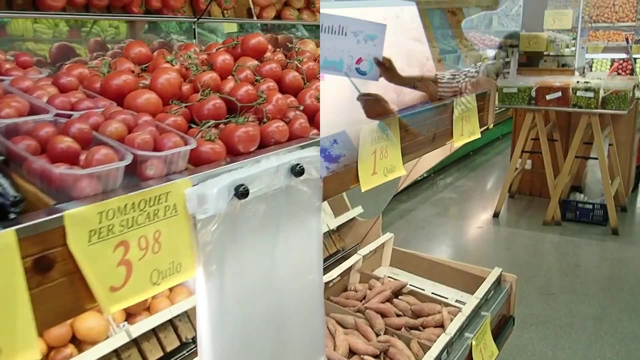 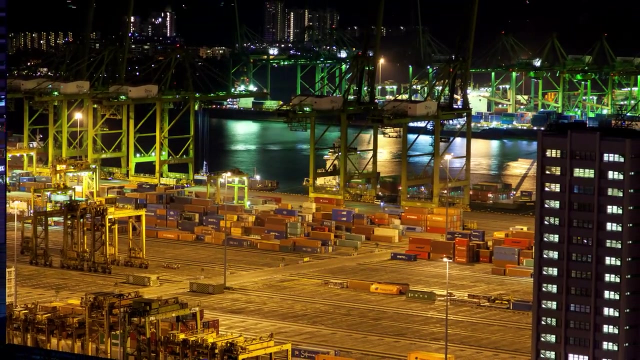 resources and transform them into a good or commodity and then distribute them to the consumer for sale. These chains encompass the entire production process, from the start where the idea is created to the creation of the good, the design, the production, the distribution and eventual sale to the consumer. This new industrialized farming is changing how we 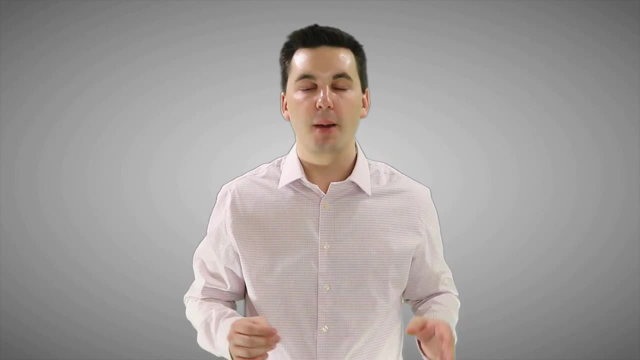 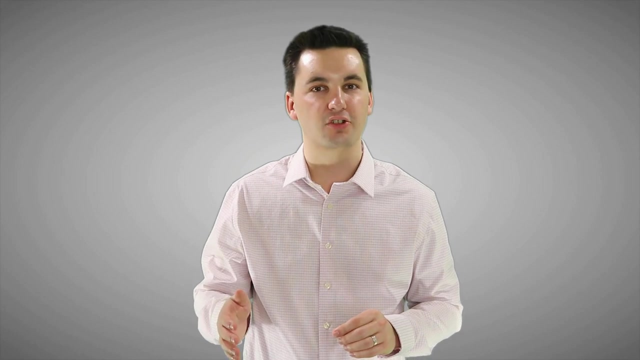 produce food. Not only now is our food being produced around the world, but we're starting to realize that we have less of a need for people to produce the food. It's changing our agricultural density, our physiological density and even the carrying capacity. Remember those? 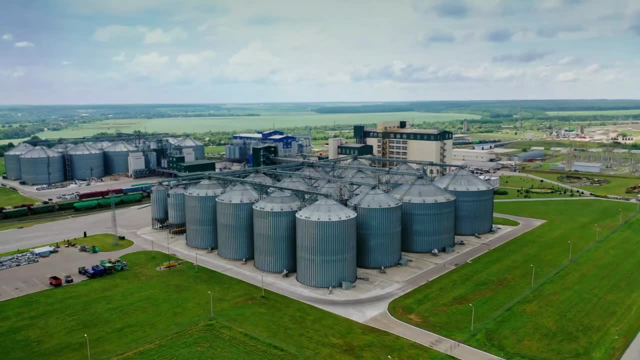 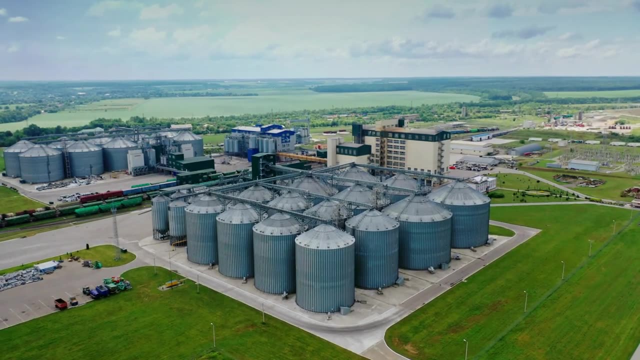 densities we talked about in our Unit 2.1 video. As industrial farming grows, so does the average size of a farm. This is because agro businesses buy up smaller farms and family farms and consolidate them under one business. These larger businesses have more capital at their disposal. 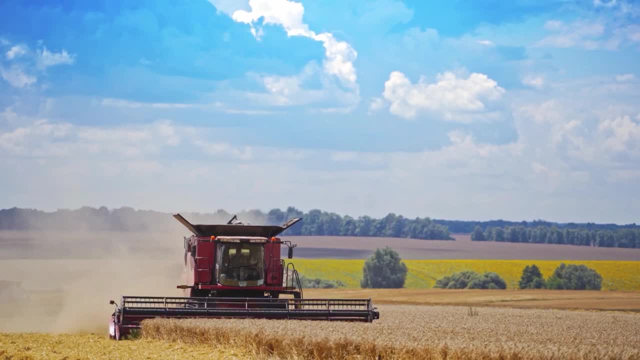 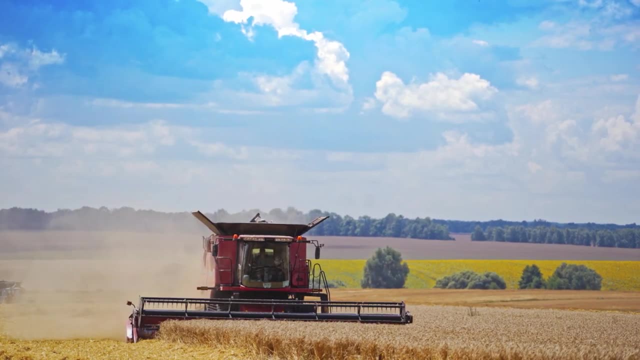 which allows for them to purchase more expensive machinery, better transportation methods, fertilizers, herbicides and pesticides. All of this allows for their crops to get a better yield and increase their profits. Speaking of profits, another way agro businesses maximize their production and also reduce.